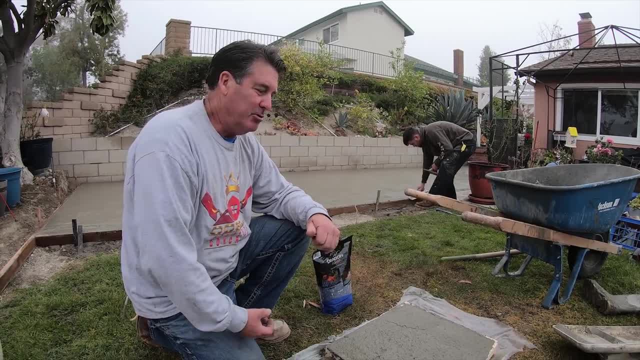 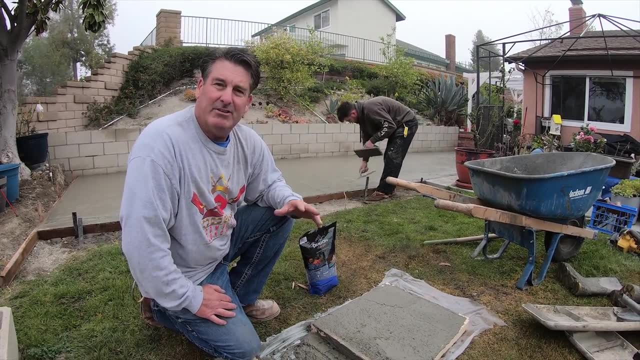 The ones that are safety glasses that breaks into the squares. That's the ones you want, but they have them and they have multiple colors. I've done it that way. Also, hit up those. You can almost get them for free, because it's all stuff that's going back to recycling, But in this case, 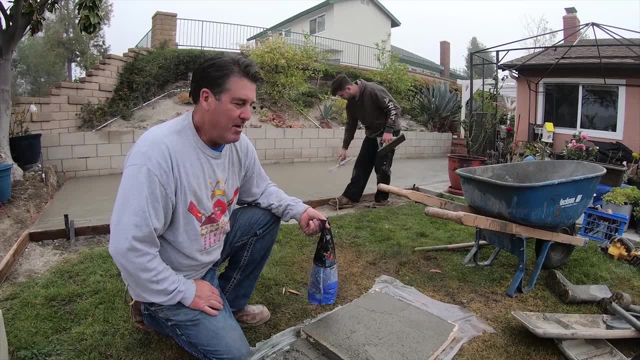 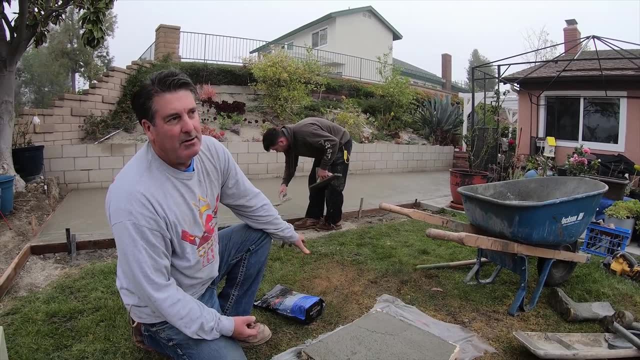 we're. this is a rush order deal. We just came up with this off the top of our head and we just went and purchased this. So here's what we're going to do: We're going to seed it, And my seeding idea with this is: I'm thinking of just kind of running some 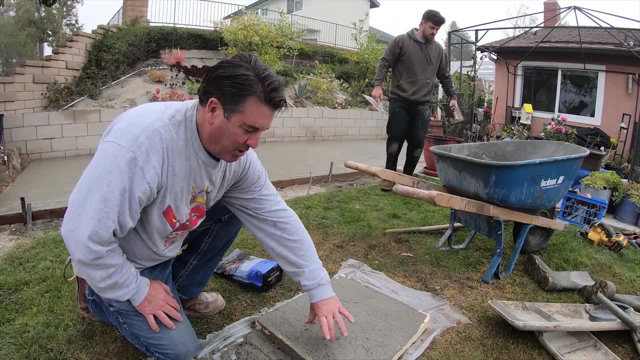 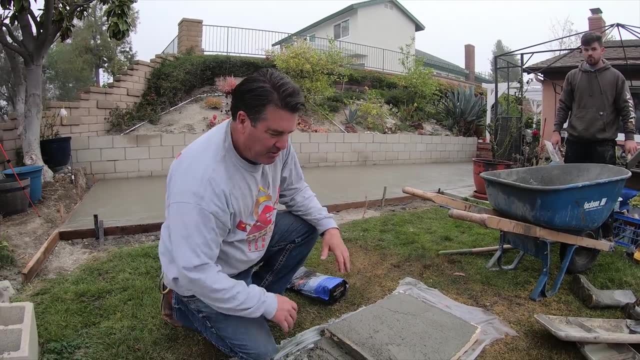 a whole thing is going to be the blue glass. I'm probably just going to run like a trail through it. I could put an O, you know, for Odell if I wanted to, or a D for David. you can do anything. 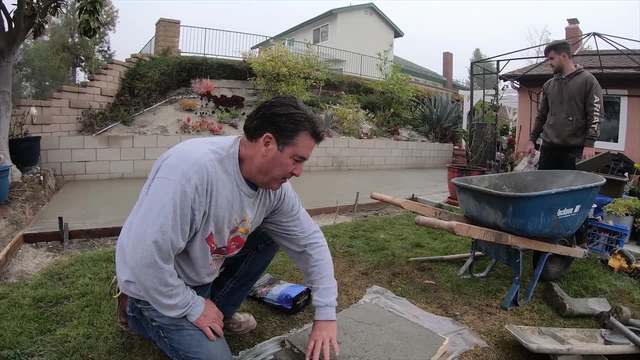 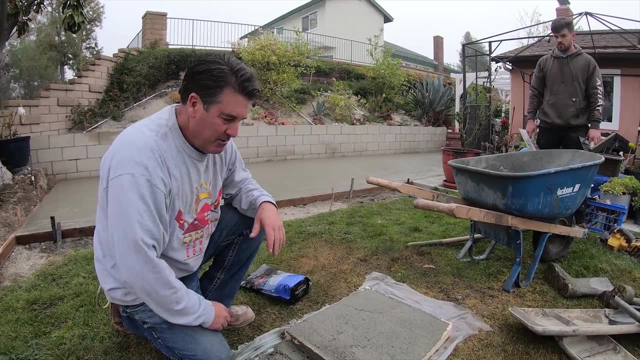 you want, You can do your own initials, but in this case I'm just going to run like a lazy river coming through here And then imagine that in different directions, entire patio with that. but we're going to show the end product and how to get there. 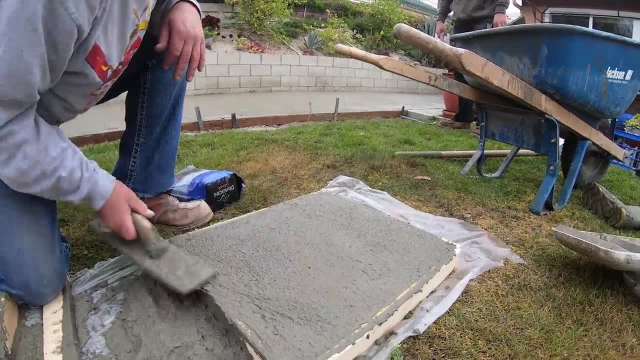 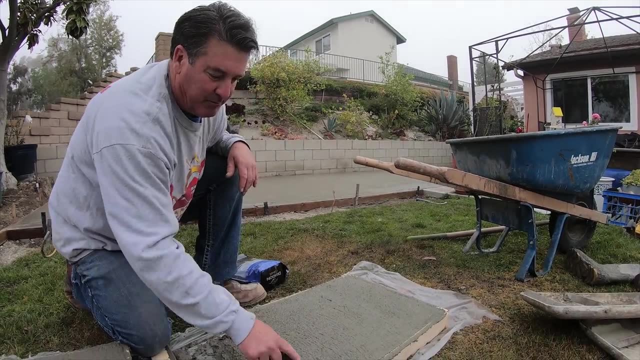 Okay. Well, one thing is to remember that whenever you're seeding, you're displacing material, So you're going to. it's going to come up somewhat like I'm at the top of form here After I get the glass in there. you know it's going to bring it up because we're displacing it. 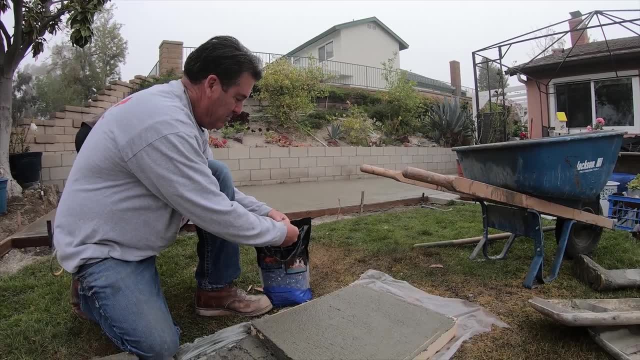 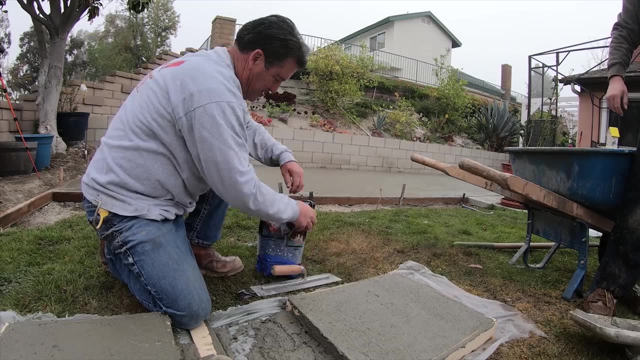 with this. whatever, however much I put in, So you may want to leave it a little low, depending on how much stuff you're going to put in there. All right, Here's what we got. Here's some of the stuff we're going to be throwing in there. 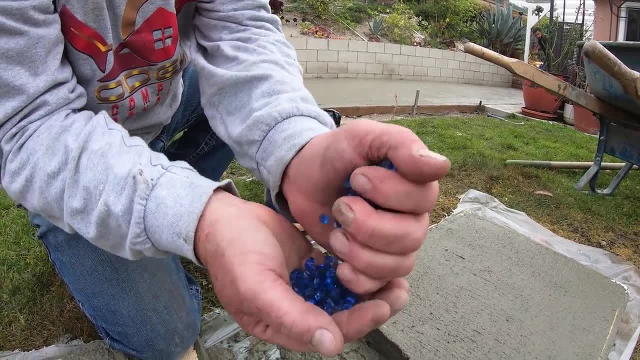 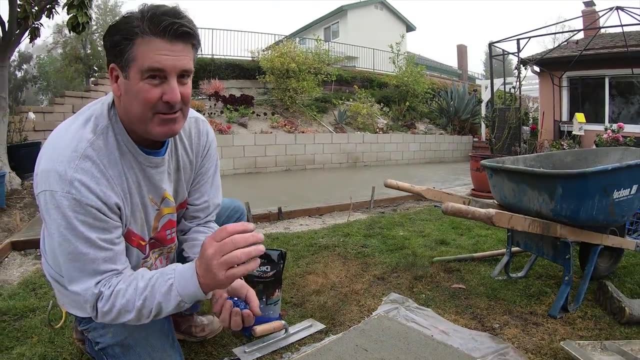 You can put rock round, rock, pretty much anything you can think of. but you know, if you did a hundred percent of this, it was nice and smooth and you had the blue glass. it might get slippery. So what you can do is either do it, you know, sparingly, you know, and separated by just concrete. 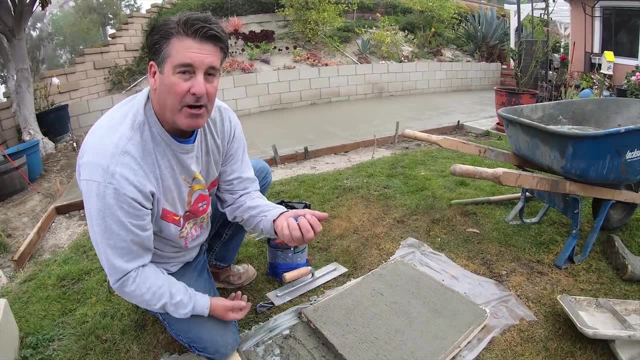 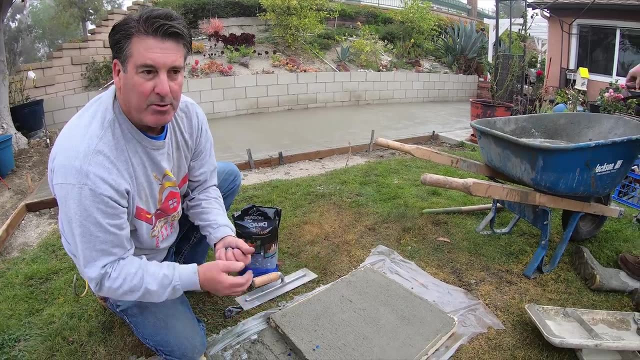 in between. So you get some traction because we're going to be washing it. So you get a sand wash with an exposure. Or you know you could put: you can go a hundred percent of this, Throw some sealer on it with a non-slip additive in your sealer, And then you know there's so many things. 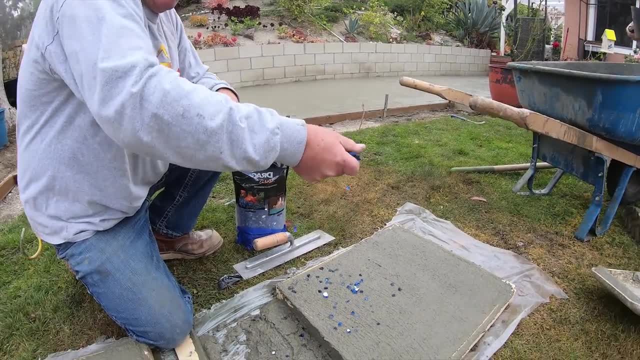 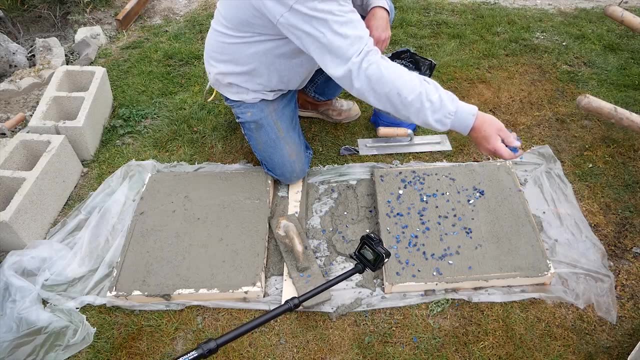 you can do. It's just just the imagination. whatever you can imagine you can do Really. That's what it boils down to Now. see how we put it on here. Not, they're not a hundred percent. This is about 50% coverage. 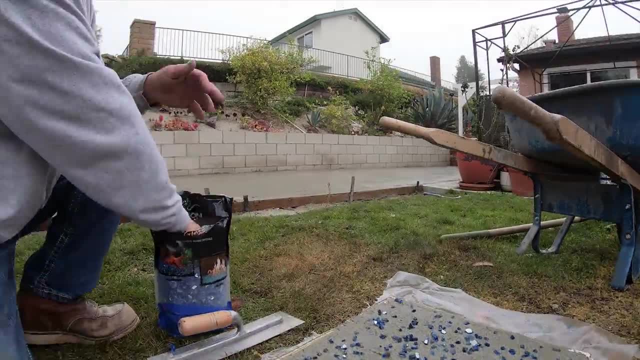 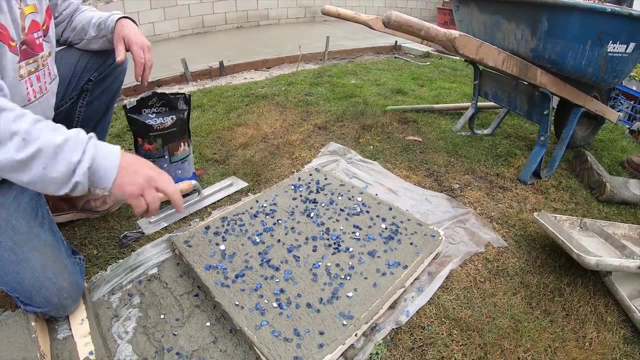 right here Is it about? feel, in your set You upstairs, could just go that route and it wouldn't be slippery because you're still going to have a sand wash texture in between these. but, um, i think i'm going to go 100 and go with the non-slip. 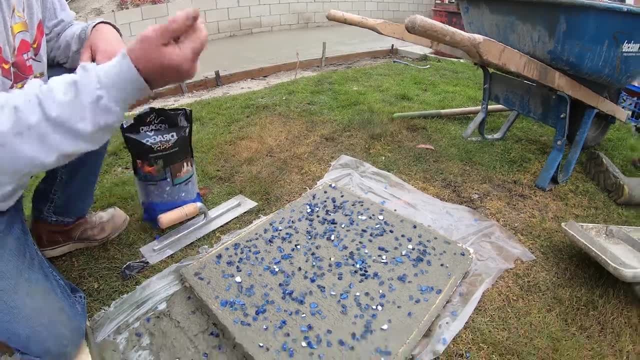 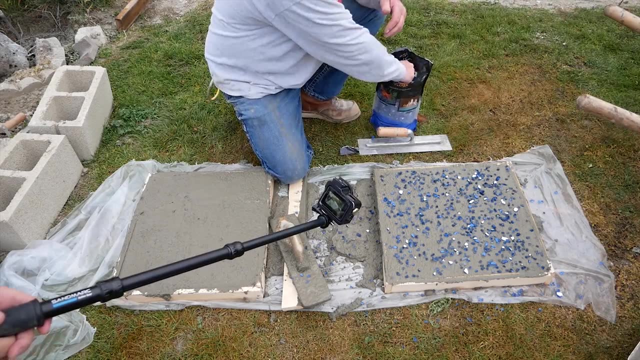 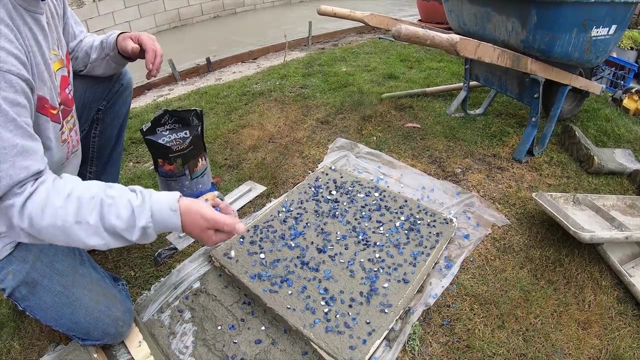 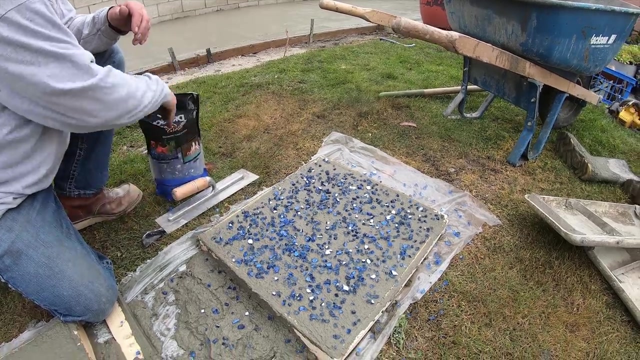 additive with the sealer, i'll go 100, maybe make this thing really pop after we do the rinse, probably, oh, about three hours we'll start the rinse process, then we'll let it cure out a few days, then we can put the sealer on. this is going to make a nice. what i'm going to do. actually, i'm going to leave this here. 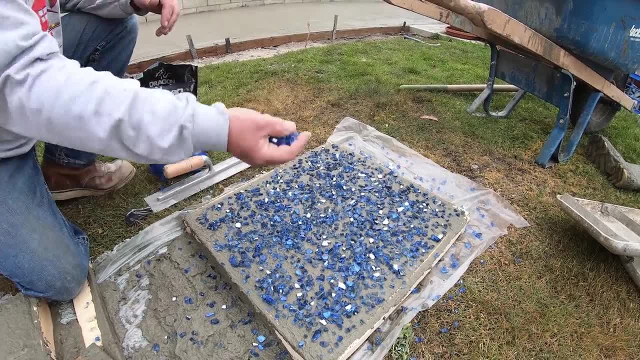 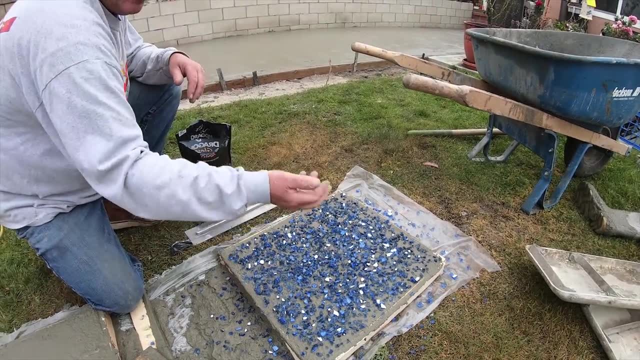 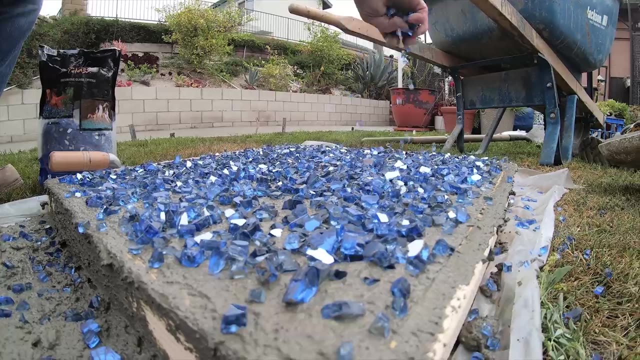 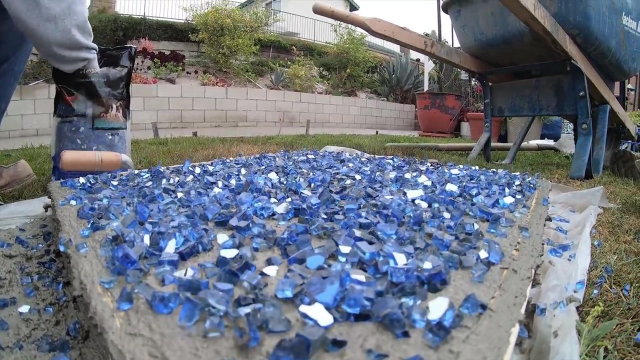 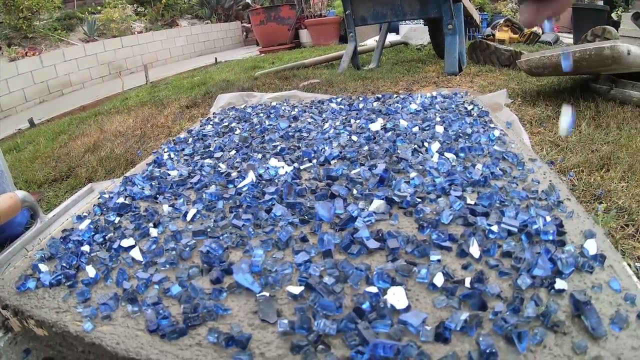 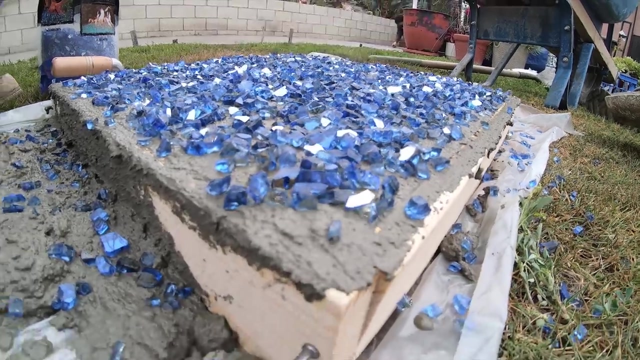 for the customer as a planter stand or a potted plant stand with 100 glass stem tape, and then i'll just put the sealer around and i will go. Eh, i'm pretty upset and i like this doing the supposed stuff. yeah, oh, that looks pretty, pretty decent, huh. 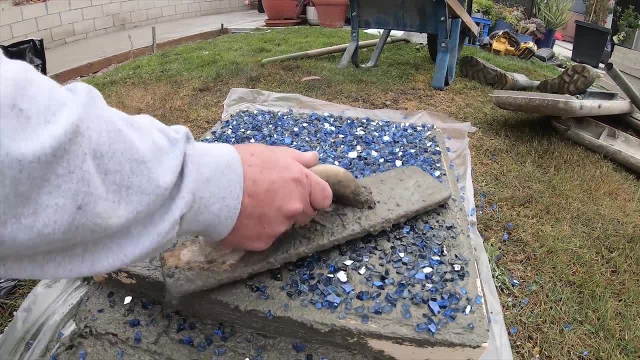 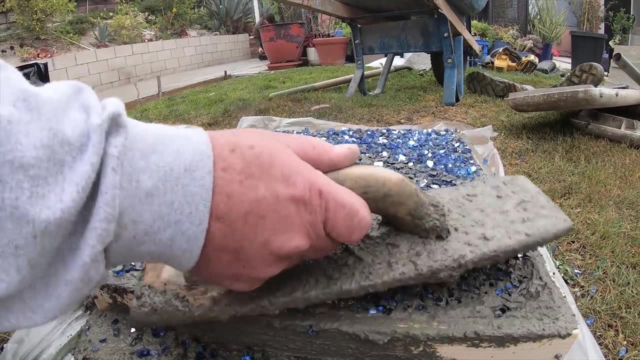 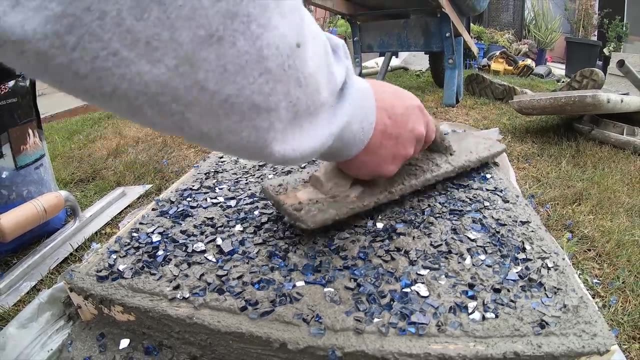 start. right in this corner, boom you to place it around the bottom of the dock, or glass in this case. you really want to get these babies locked in, so you've got to get 100% coverage around every piece, otherwise they're gonna come out later if you don't. 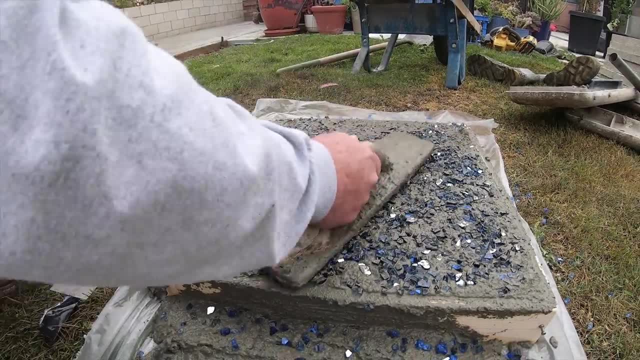 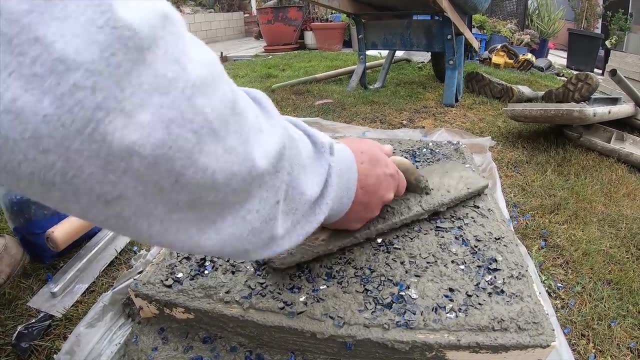 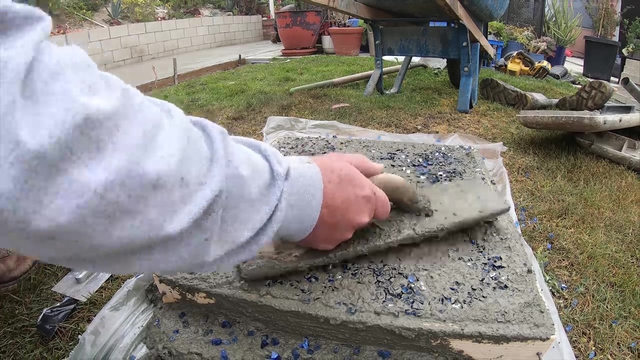 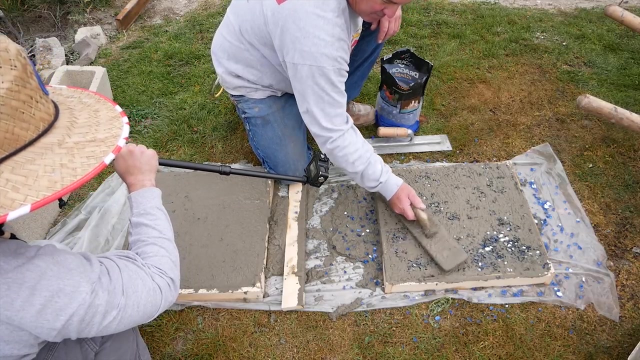 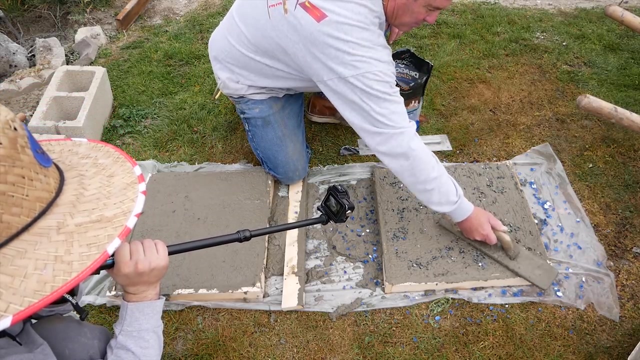 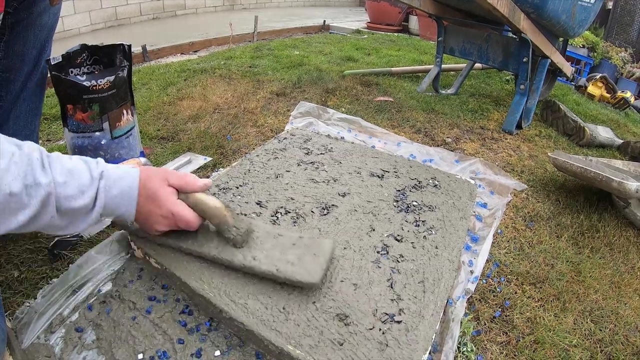 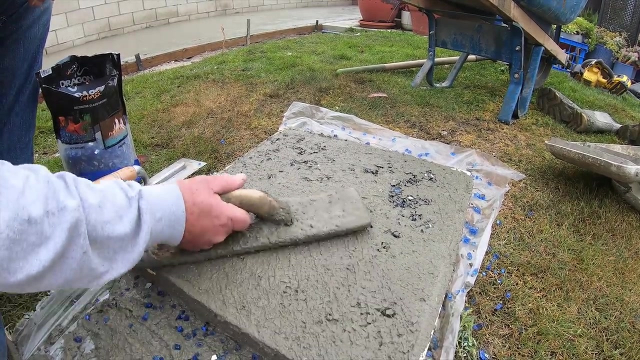 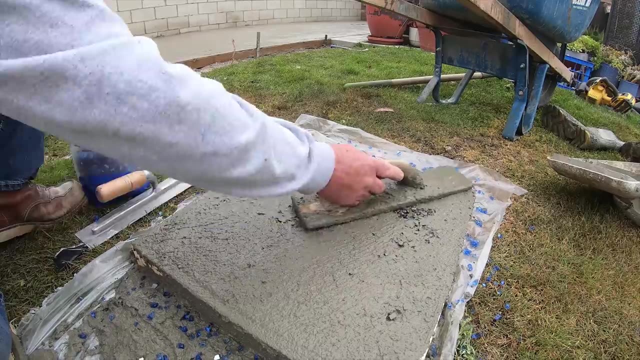 get that cream to come up. just keep beating it until the cream rises, almost disappearing. now, once it's disappeared, you gotta let it set, maybe trowel it, throw an edge on it. you know, in this two and a half hours we have to work with, go eat breakfast, come back, toy with it some more. 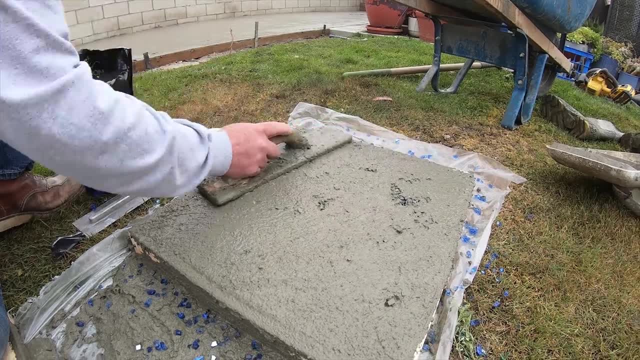 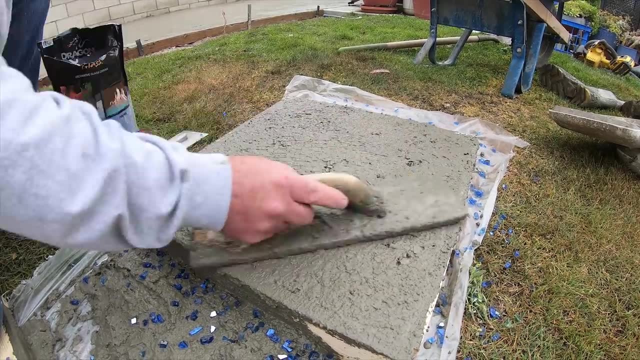 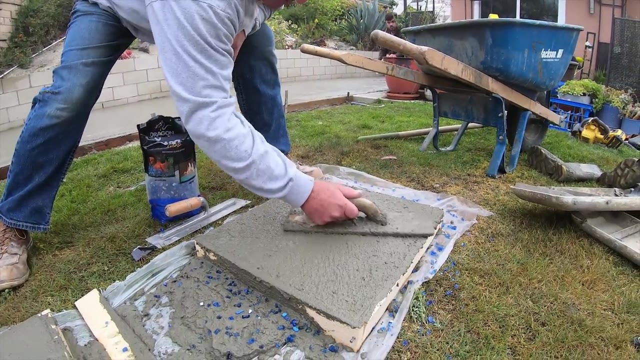 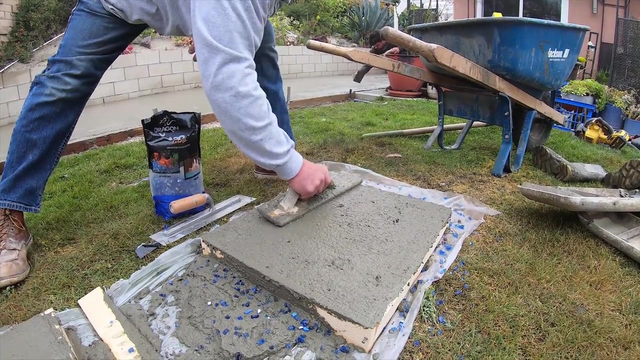 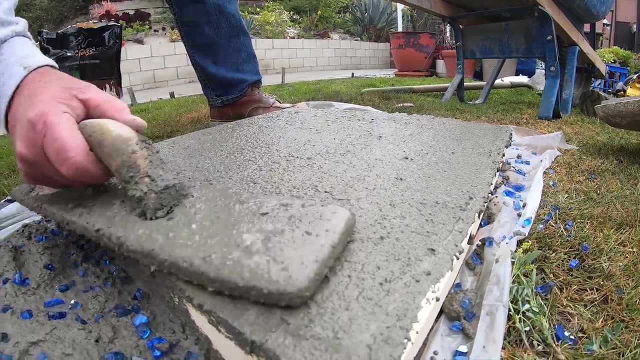 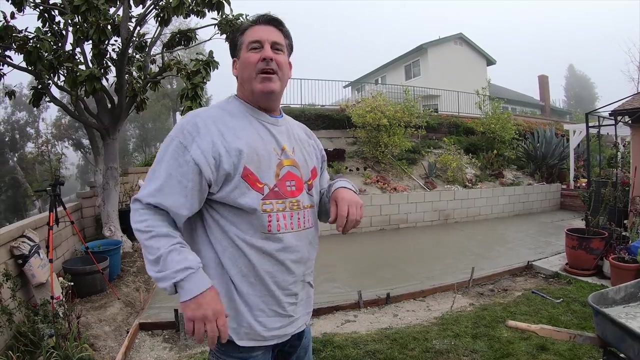 it's all gone. no one would ever know it's in there now at this point. okay, that one's ready. we'll catch an edge on that a little bit later. we don't want to edge it early. if we edge it early it's gonna roll the edge, you may. 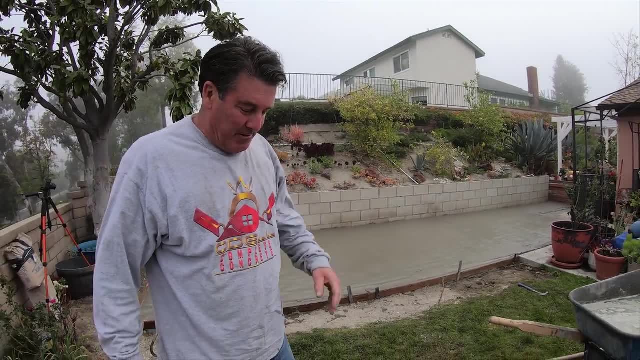 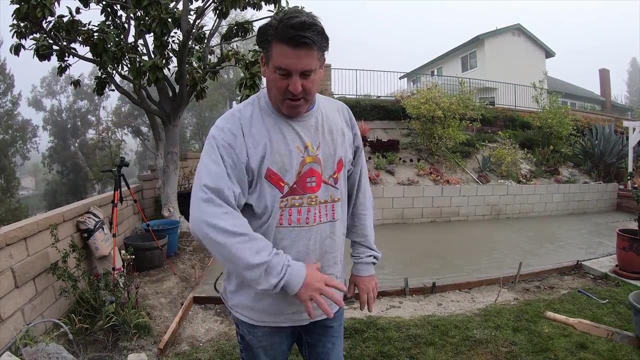 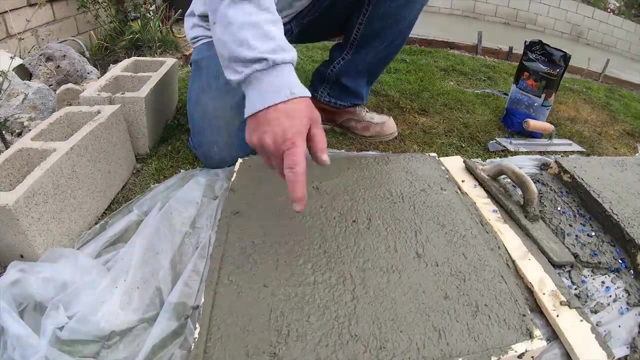 get the glass too deep, then it's harder to expose. so let's move on to the next design, this one, I think we'll just do a, let's just do a little trail going through it. now let's put, let's put- an O on it. yeah, you put an O, so the O could. 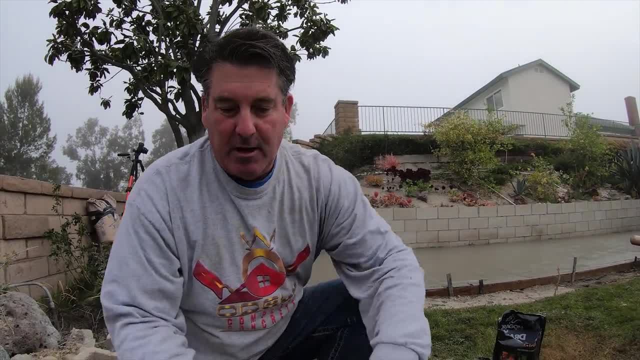 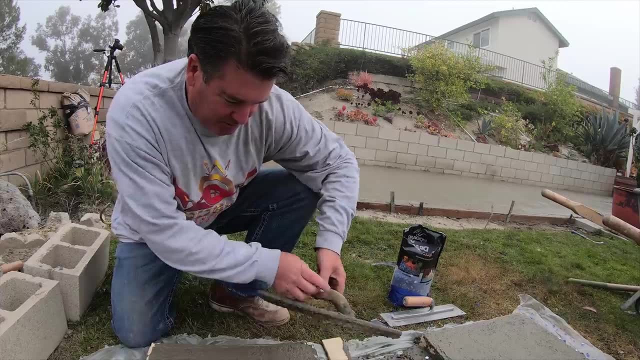 be a couple things. it could be a little bit of a little bit of a little bit of a little bit. you can be the center of where a pot would go, or, you know, it can be a my initial, like Odell, but we'll just do an O. 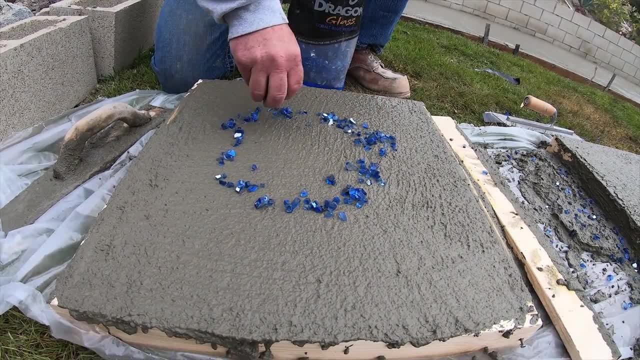 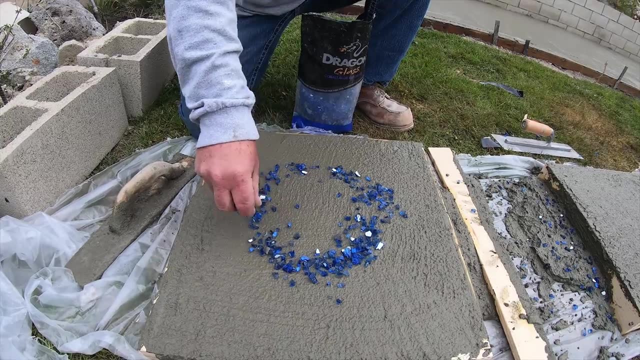 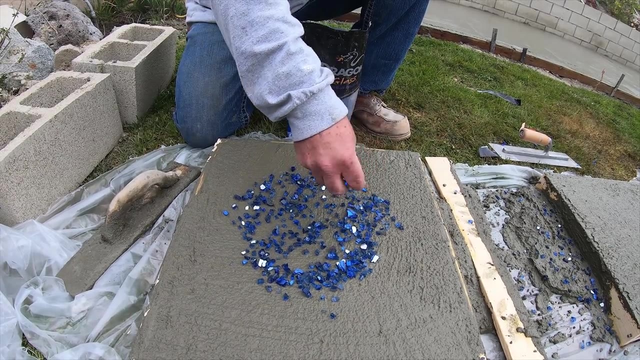 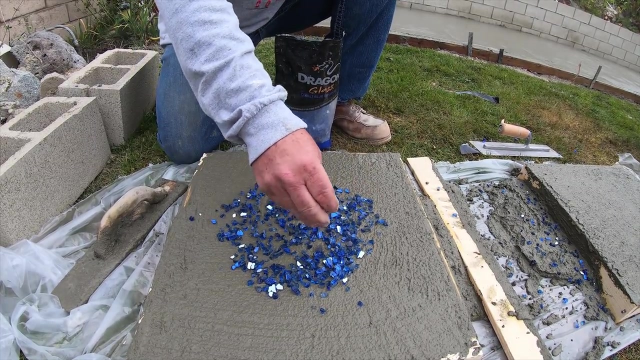 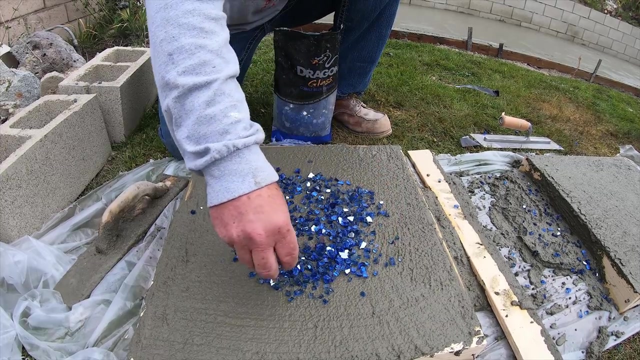 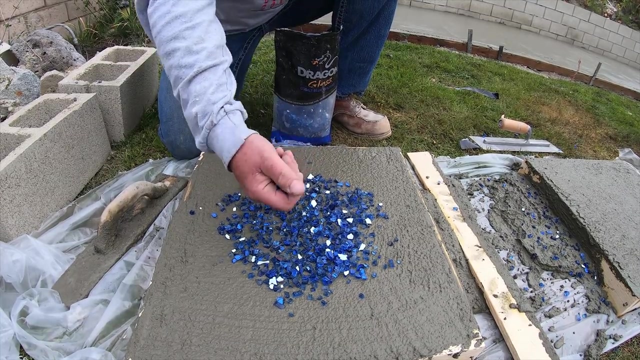 we'll do a solid circle right in the middle. yeah, I don't really. I've really don't get this. actually, you know, before I did a lot of seeding with rock and other things but always wanted to do the glass. what if I just do a couple shards going out? 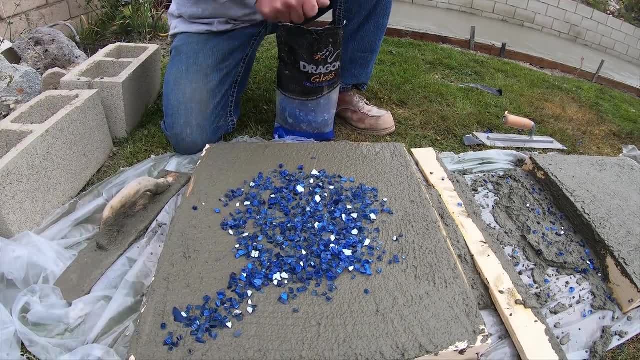 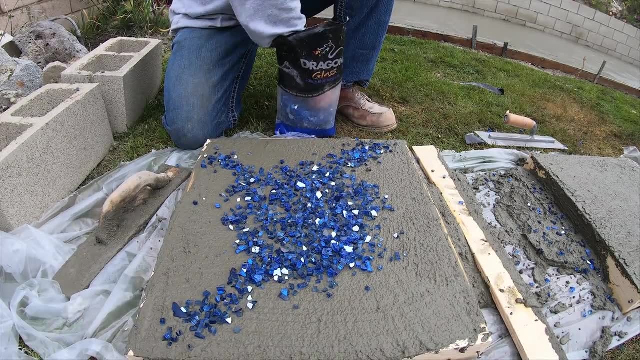 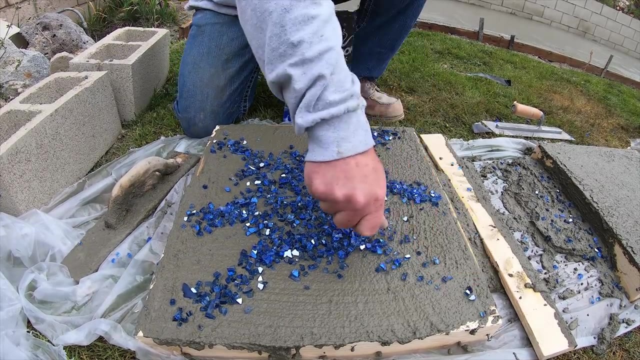 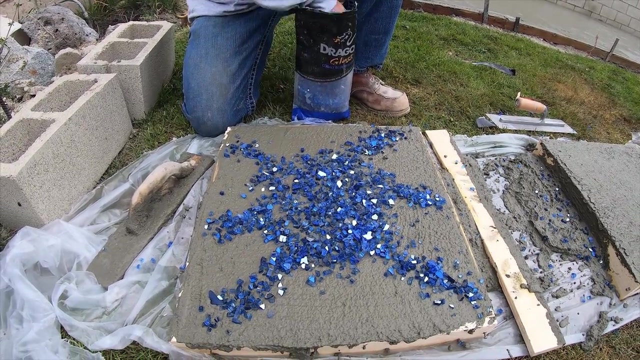 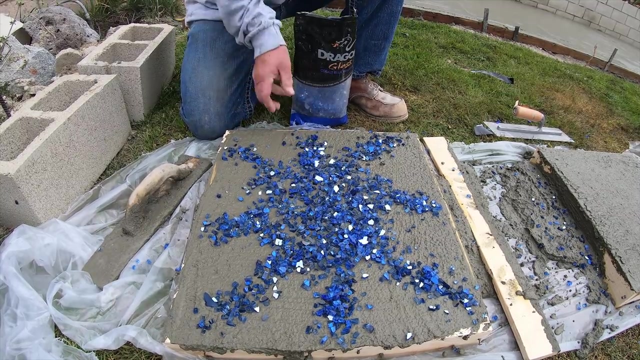 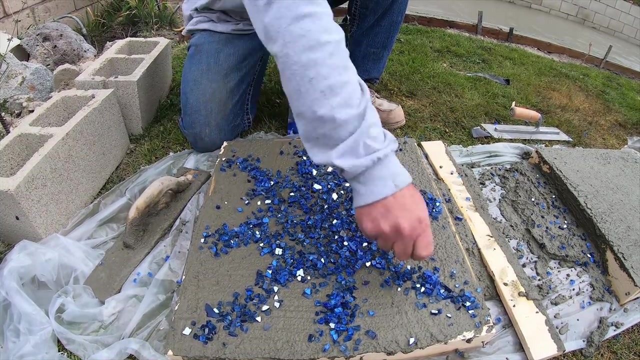 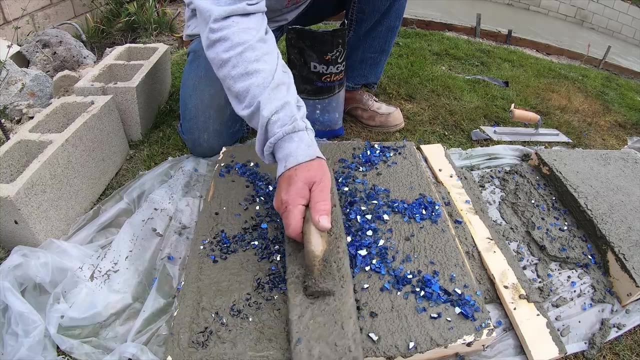 like a sun ray or something. last a couple pieces going out from this, shards going out of this like a burst. you pretty good, huh? just see what that looks like in the end. yeah, it's pretty cool. pound it in and see what happens. trying to keep that glass. 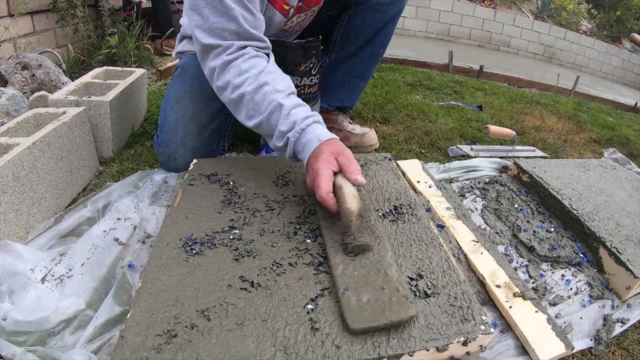 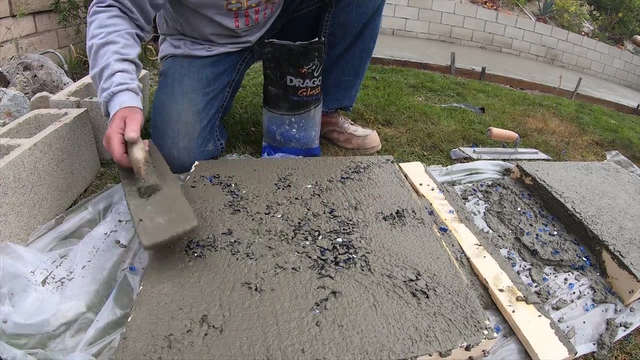 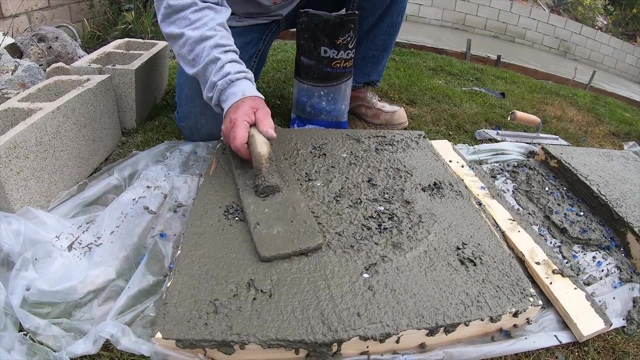 pretty much where I set it. I could smear it all the. I could smear it all over the place and then we wouldn't have whatever pattern I use would be kind of dissipated. but try to keep it right where I put it, mostly by setting it straight down by 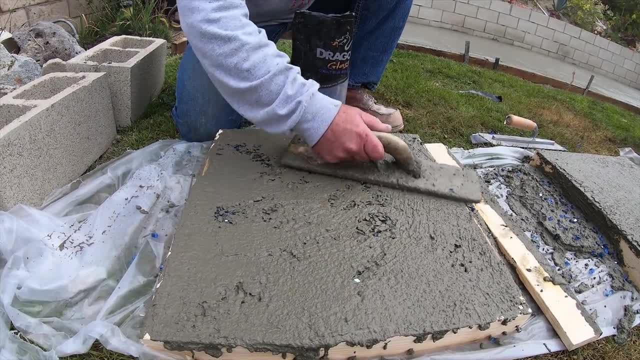 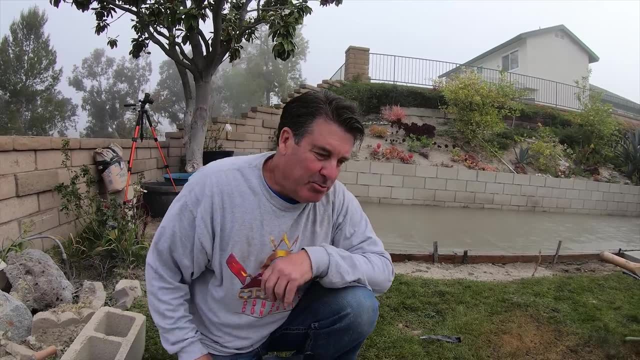 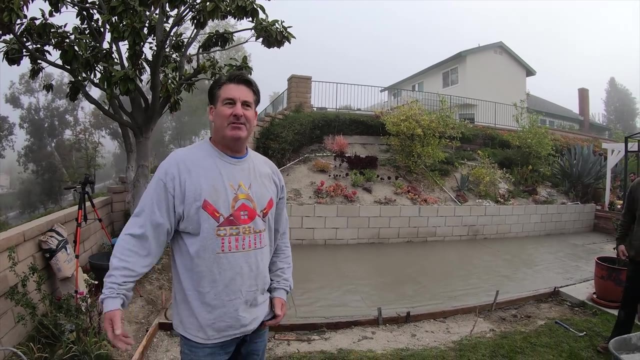 tapping it and it won't move as much. there it is, let it set for a while. don't want to overwork this, don't want to get it to recess, so we're gonna minimize the work time on this. keep everything up so it's easy. rent less material, take off. 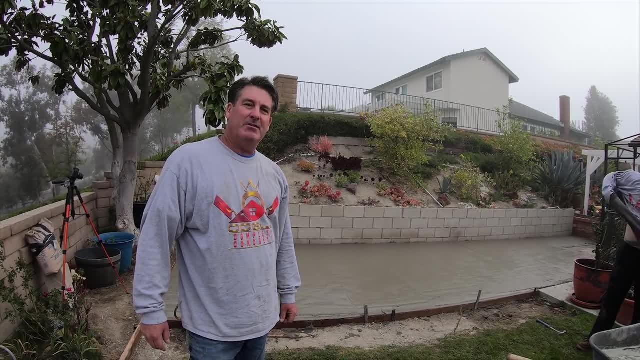 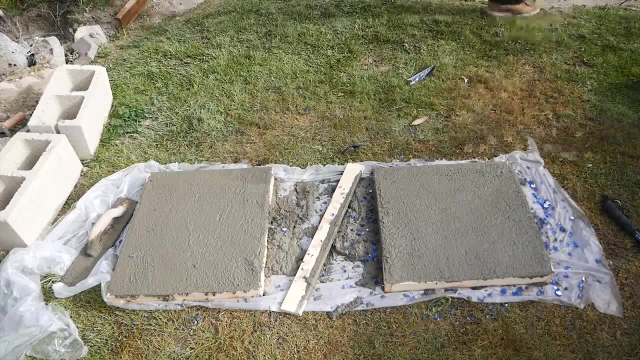 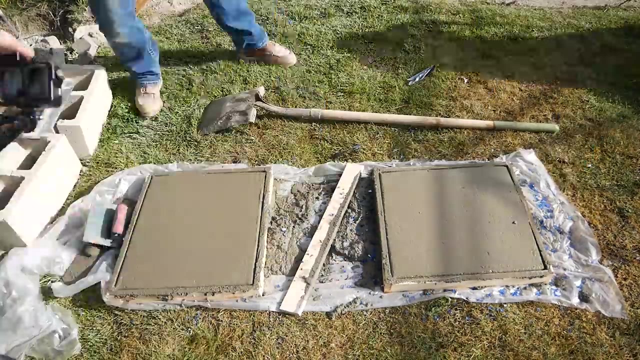 the top. all right, let's get back to the main job site. this is just a little fun thing I'm just kind of doing for the DIYers out there. okay, so this is the first time we're gonna work the concrete. what we've done. we just we did the hand. 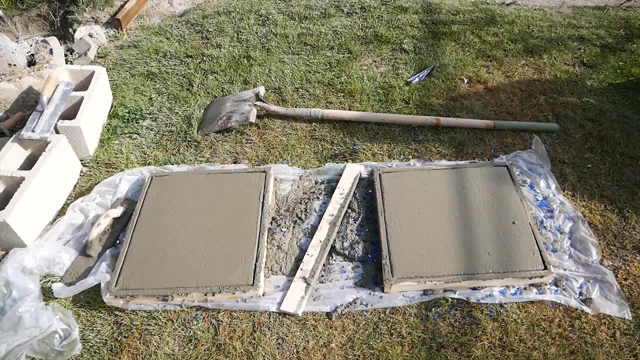 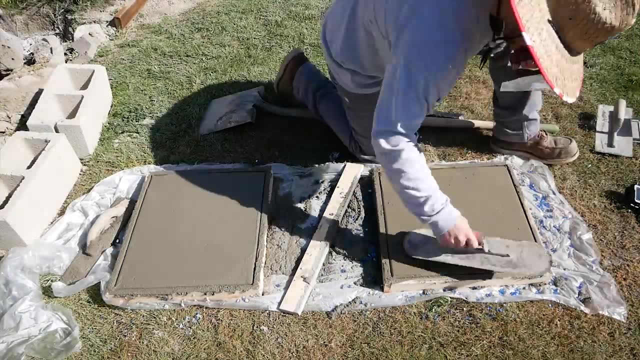 float embedding the glass beads, and then we let it set for a while. we let it set approximately one hour before we touched it again, and then we went ahead and started putting the steel to this an hour later, which was the hand edger and a trowel. 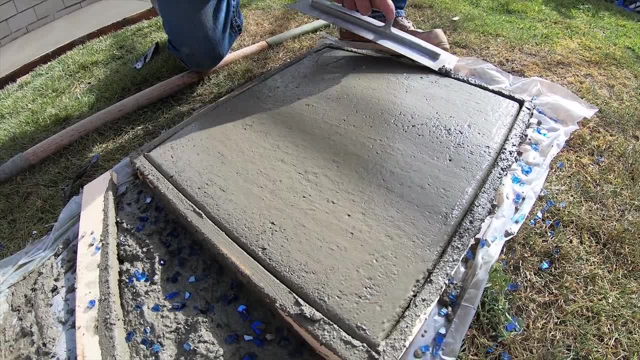 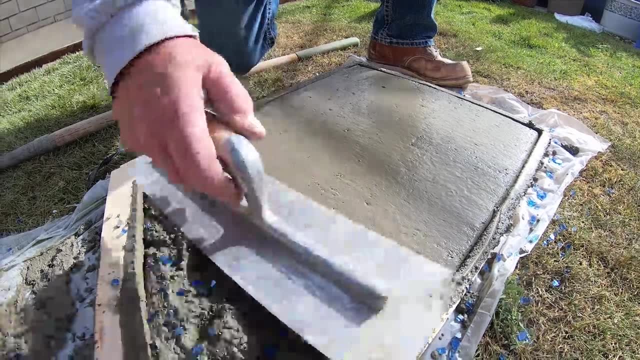 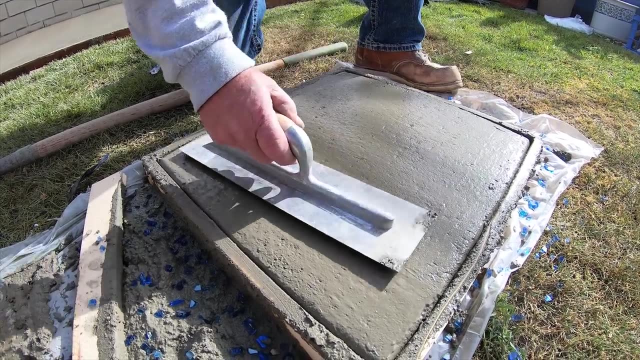 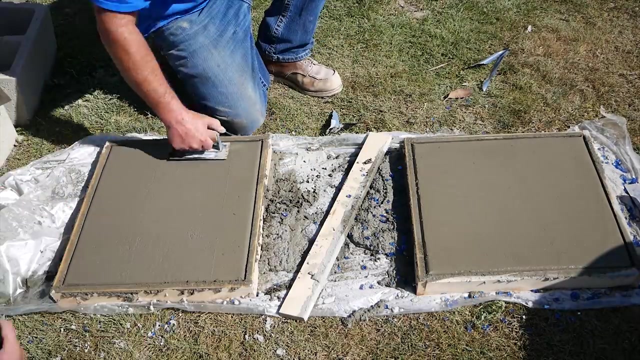 that's a six inch wide, half inch radius hand edger and the trowel is a 14 or about a 14 by 3, that's an 18 inch square. so you can see the glass kind of popping there. and the reason it does that is because the cognates really not hard. 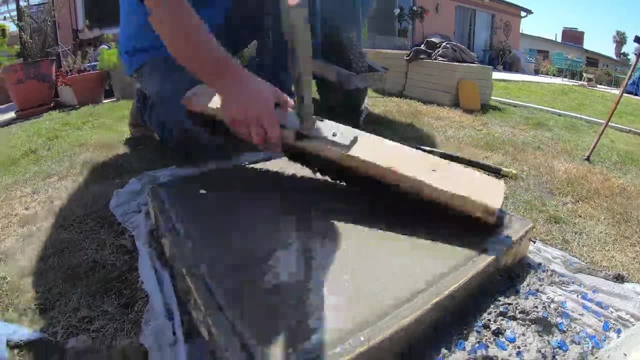 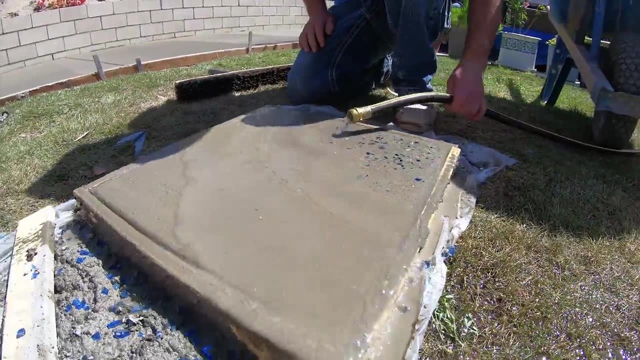 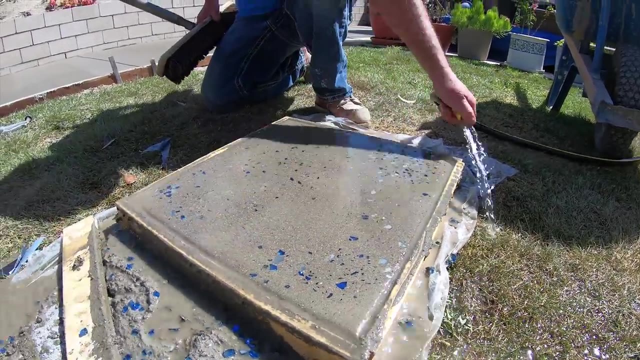 enough. so the glass is gonna keep trying to roll over on you as you trowel it. so, as it gets harder, the next time you trowel it you won't have to worry about that glass popping. now, right here, the concrete that we poured the actual patio that's already completely finished, broomed and 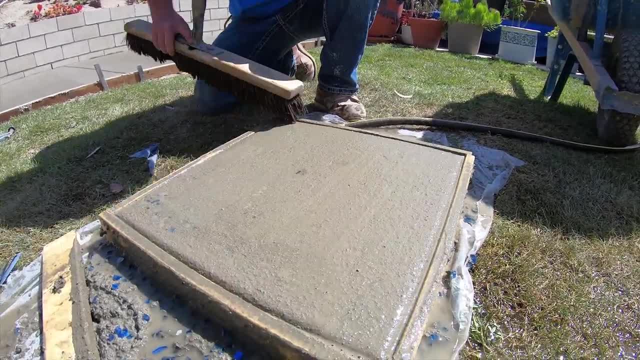 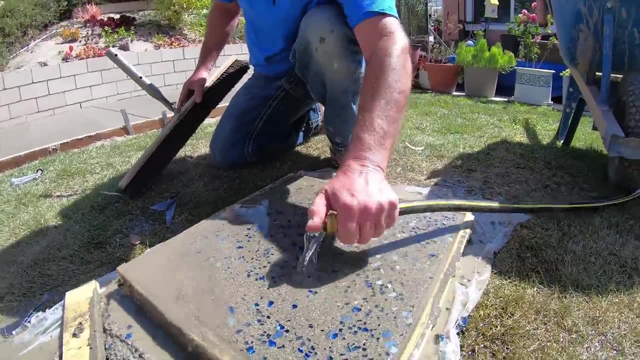 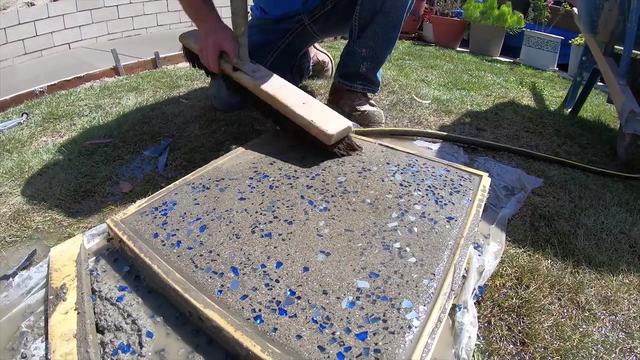 we waited an additional 30 minutes, so we're already into this stepping stone about three and a half hours at this point. when we started rinsing- and the reason we're waiting longer on this- then we did for the typical broom finish that we did on the patio with the same concrete load is because we just 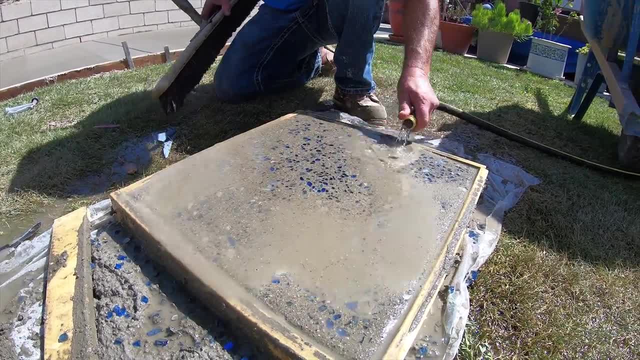 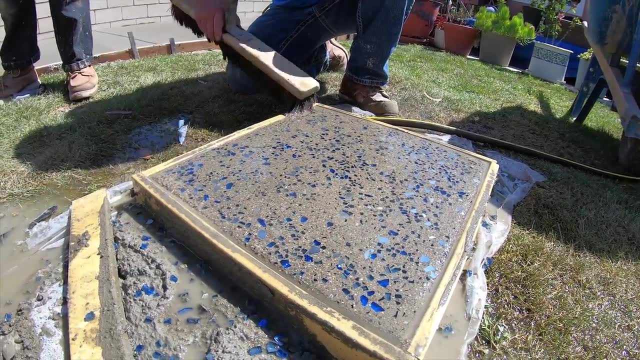 want to take a very little bit of the surface off just to expose the glass now. if you rinse early, you're going to get pits in it and you really can't fix it at that point. so it's better to go late and use a little more elbow grade elbow. 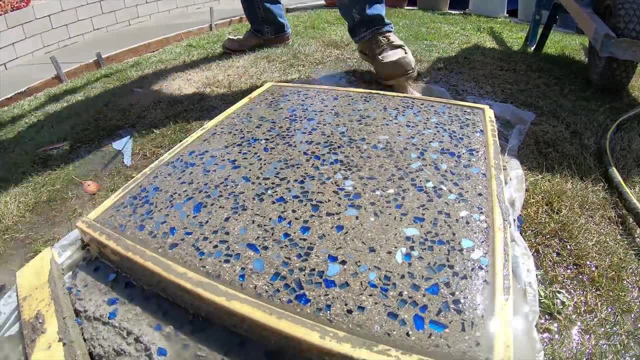 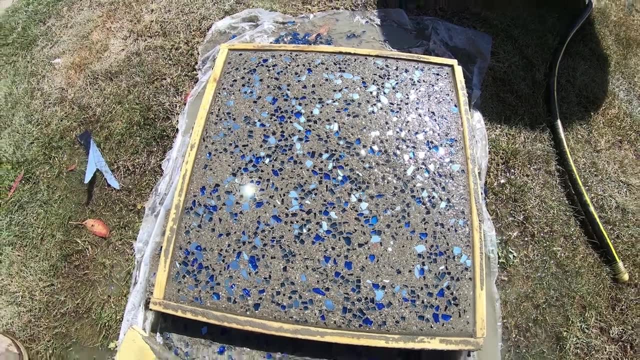 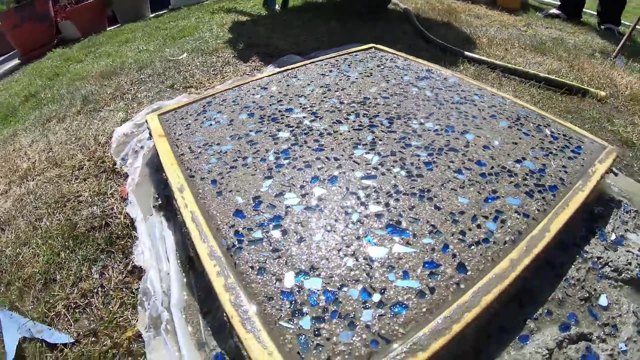 grease rather than not going early, because once you go earlier in your in trouble. also, if you notice, I didn't use any kind of a nozzle on that water hose. we just let it came out. come out of the water hose, naturally, no pressure, just let the water flow over it. loosen it up with a horsehair nylon mixture. 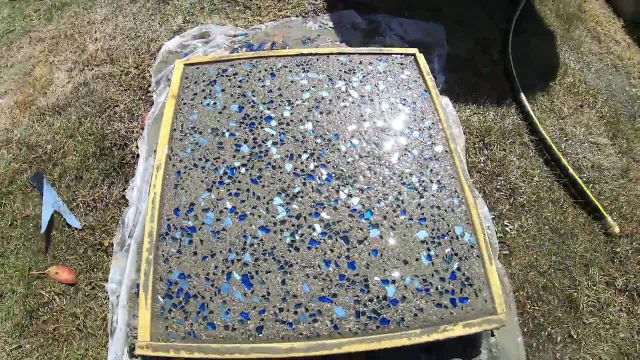 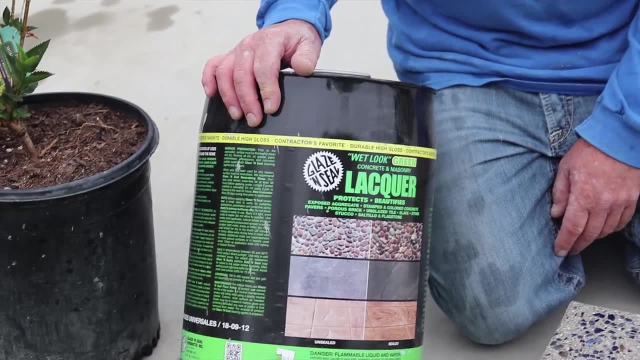 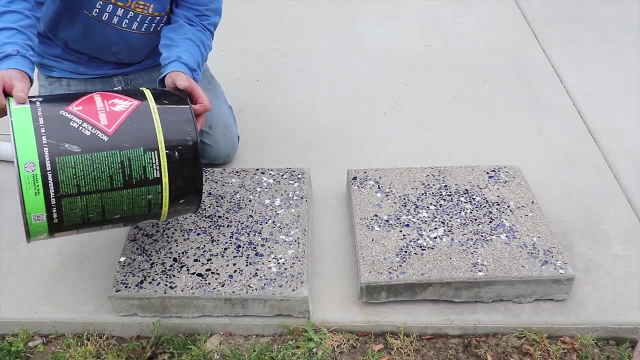 broom, real soft broom. if you use a hard broom you're gonna start popping those glass beads out, so you got to use soft texture broom to do your rinse. here's your sealer. we're just using that glazing seal readily available at Home. 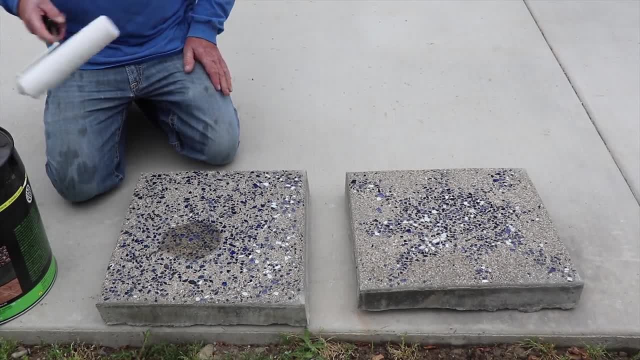 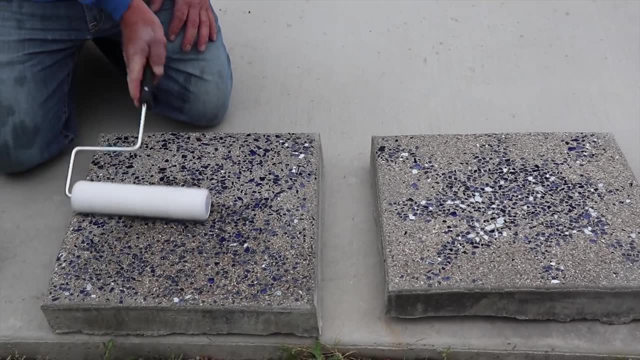 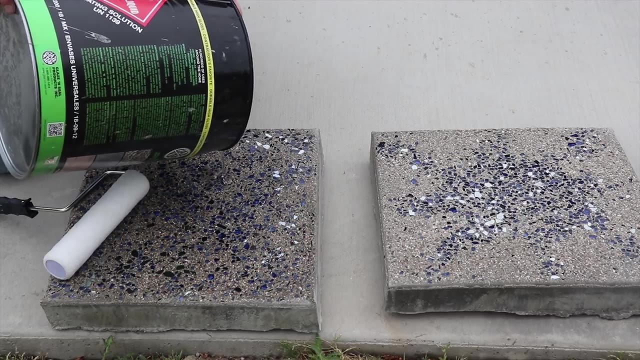 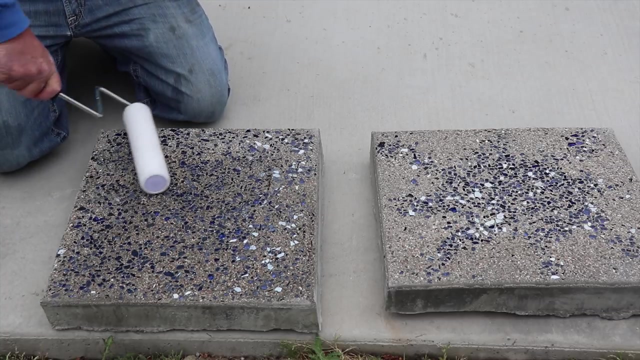 Depot because of the low VOC and that means that, as it dries, the emissions from it it's very minimal. so you're really taking care of the climate by using this particular product. and what the sealer is gonna do by selling this: it's gonna maintain that nice shiny look and it's gonna look wet all the time. 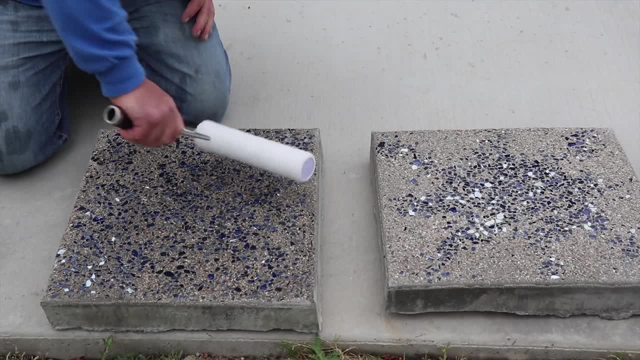 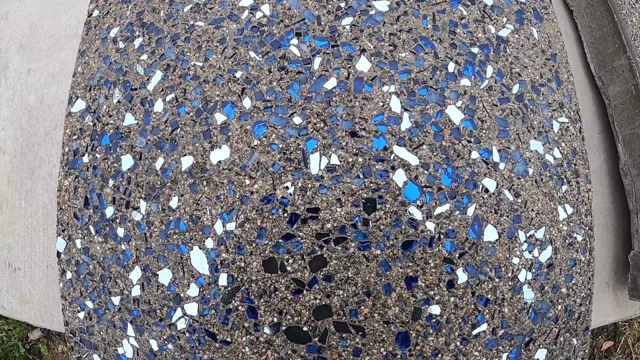 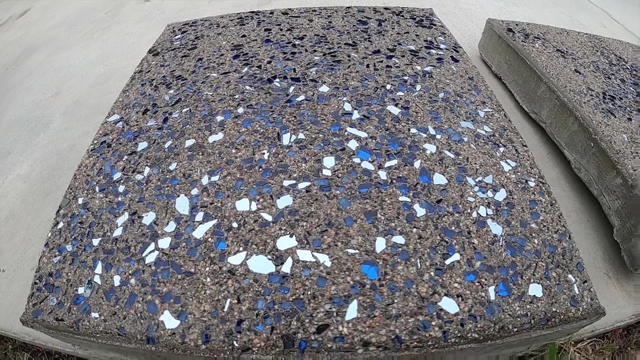 also, it's gonna prevent staining, like if you put potted plants on this and the leaf water running out from the pot of plants could stain typical concrete. with this sealer, that'll protect it so it's easy to clean. in the future. you just probably need to reseal about every five years. all right, that about wraps up this.